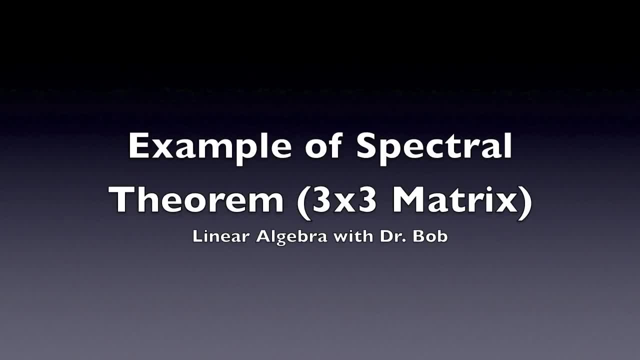 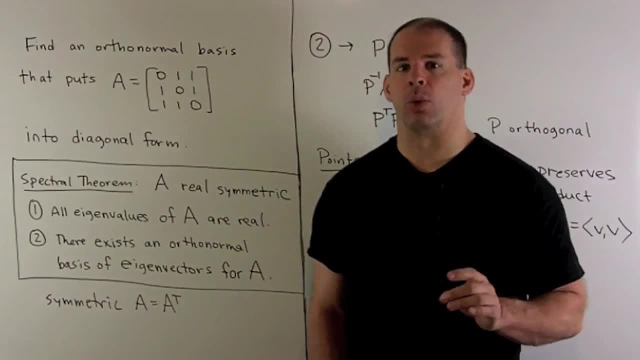 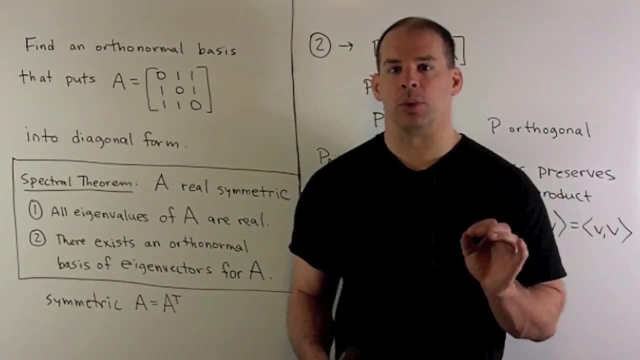 Find an orthonormal basis that puts the following matrix A into diagonal form. Now, A is going to be the 3 by 3 matrix. Every entry is equal to 1, except along the diagonal, where they're equal to 0. Our problem is going to be an application of the spectral theorem, So we 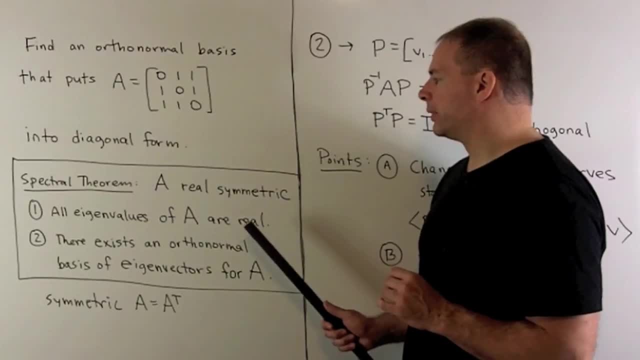 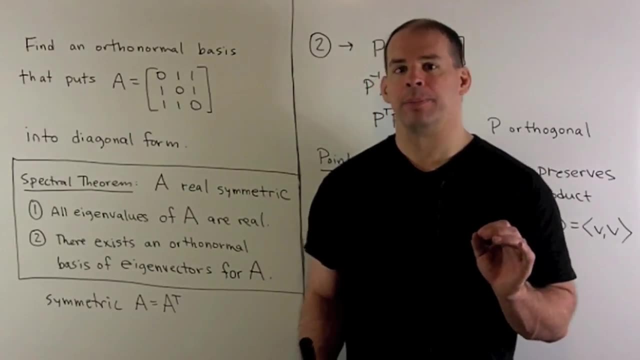 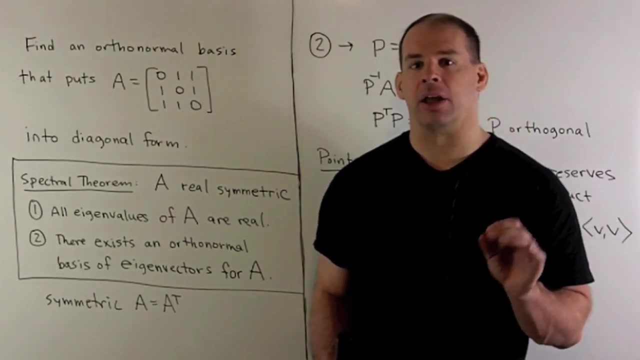 have. A is a real symmetric matrix, so all the entries are real. We take the transpose of our matrix, we get our matrix back, Then all the eigenvalues for our matrix are going to be real and we're going to be able to find an orthonormal basis of eigenvectors. 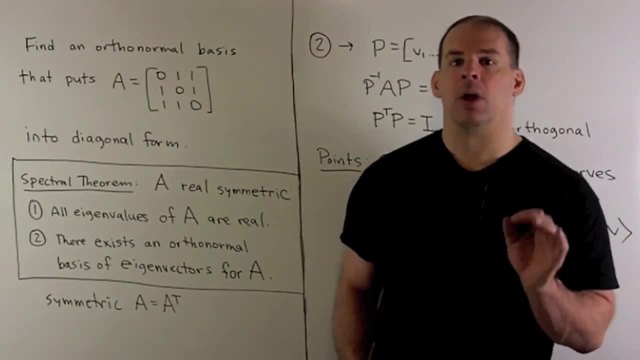 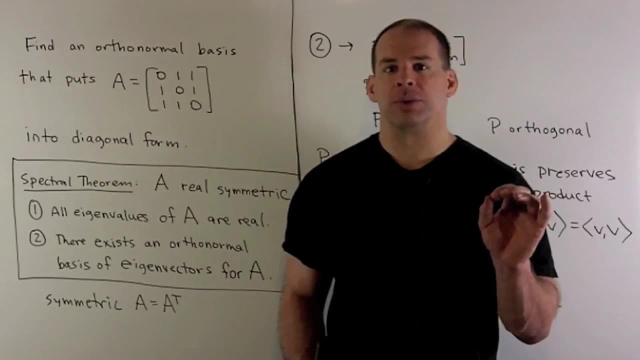 for our matrix. Now, why is this significant? Well, if we take any real matrix, if I go looking for eigenvalues, I'm going to be able to find an orthonormal basis of eigenvectors for our matrix. So if we take any real matrix, if I go looking for eigenvalues, we're not 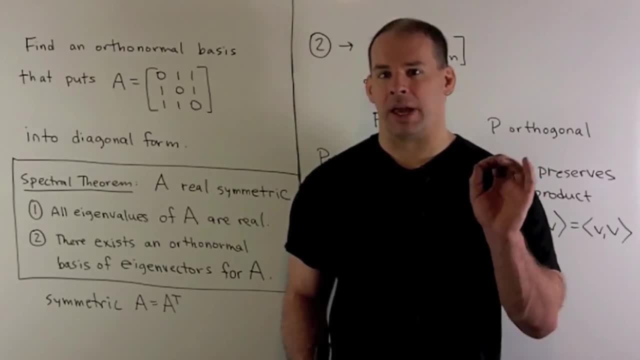 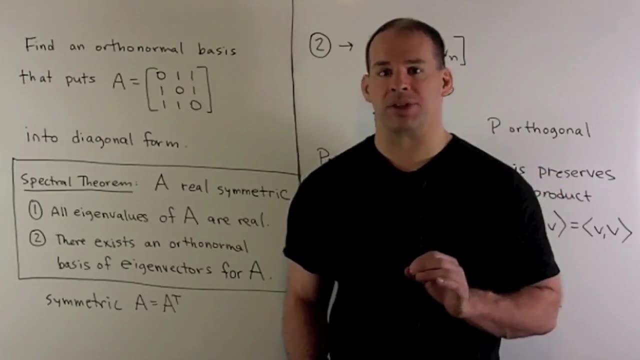 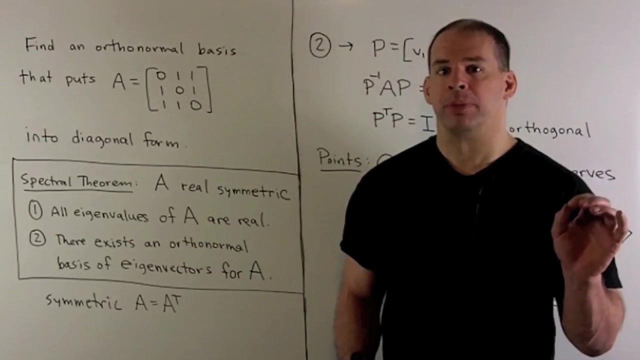 guaranteed that they're all real, So we could wind up with complex numbers. If I want to stay in the context of real vector spaces, we can't use complex numbers as eigenvalues. Then even if we have all eigenvalues real, there's no guarantee that I can get a basis. 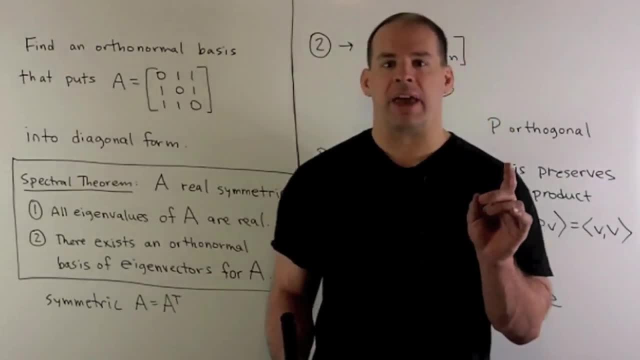 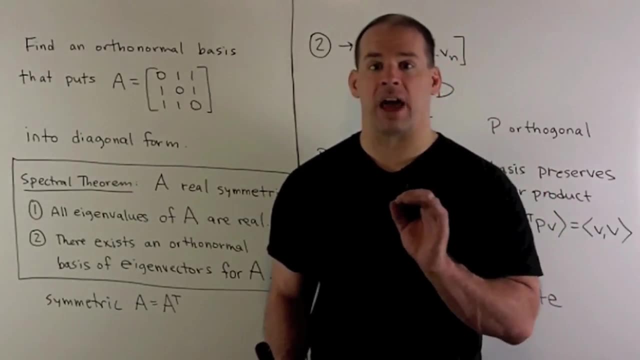 of eigenvectors. So what happens there? you're going to need to forget about putting your matrix in diagonal form, and then you'd want to try to find an orthonormal basis of eigenvectors. That's why you want to do something like, maybe, Jordan canonical form. Okay, Now note to 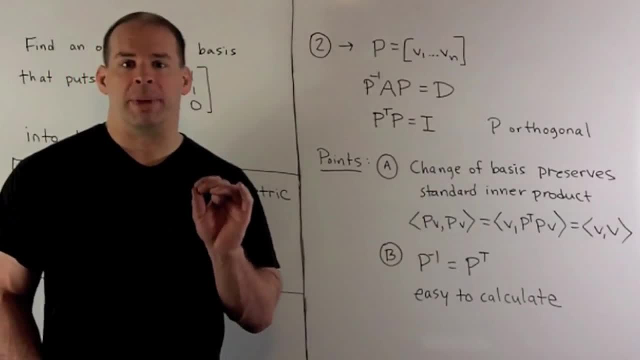 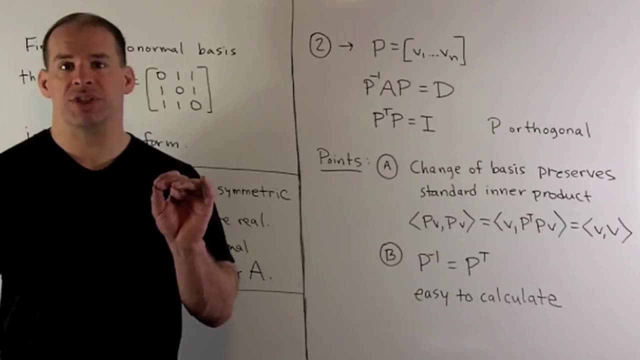 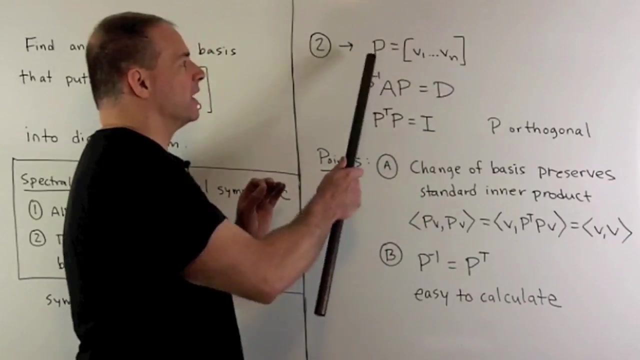 say that I have an orthonormal basis of eigenvectors. okay, well, that just means if I take those eigenvectors and I form the basis matrix, so we're going to take our vectors, put them into the columns of the matrix, then this matrix will put A into diagonal form. Okay, 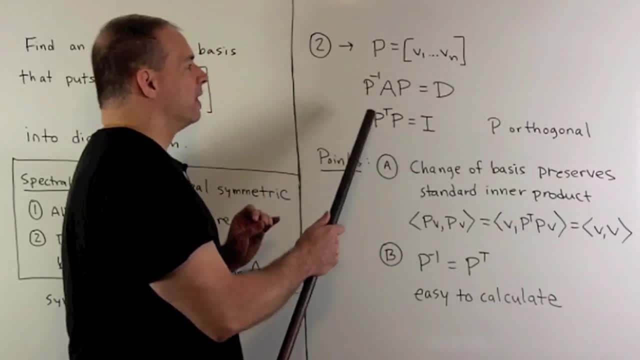 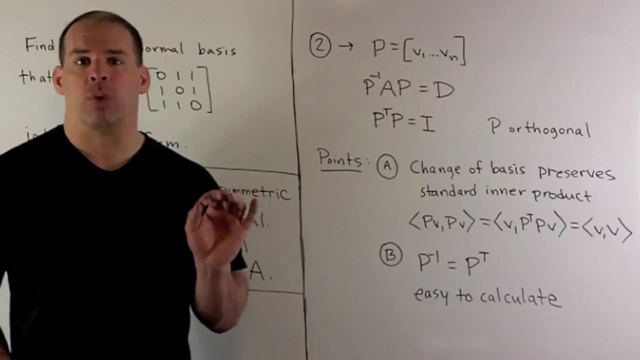 so D will be diagonal. Okay, so this matrix will put A into diagonal form. Okay, so D. and then we have that. if I take P, transpose times P, we get the identity. So we're able to put our matrix in diagonal form using an orthogonal matrix. 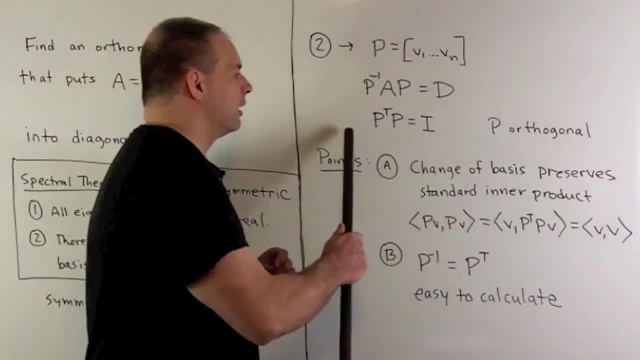 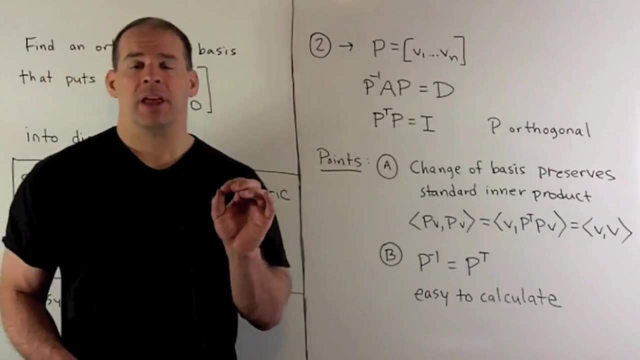 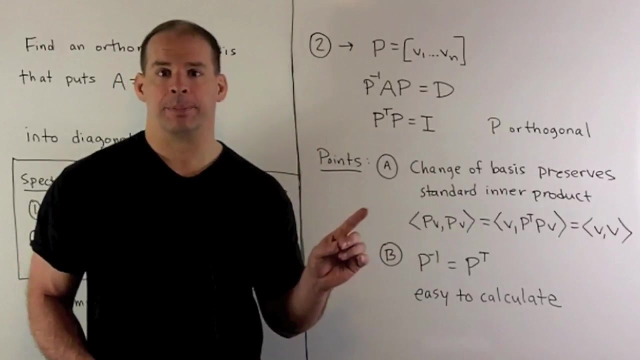 To give an idea of what this equation here says, if you work out all the row-column products, that's just saying columns are orthogonal if they're not equal and they're going to be unit vectors if we measure the lengths. Now what's the point of having an orthogonal matrix? 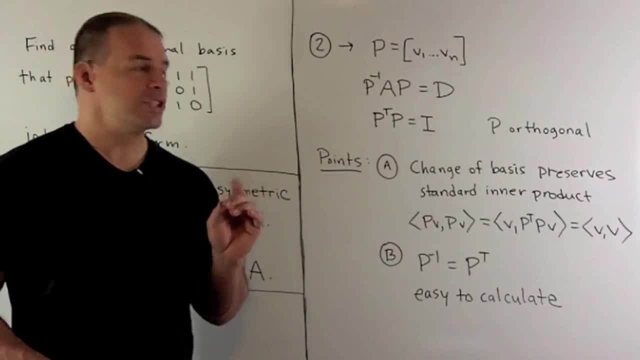 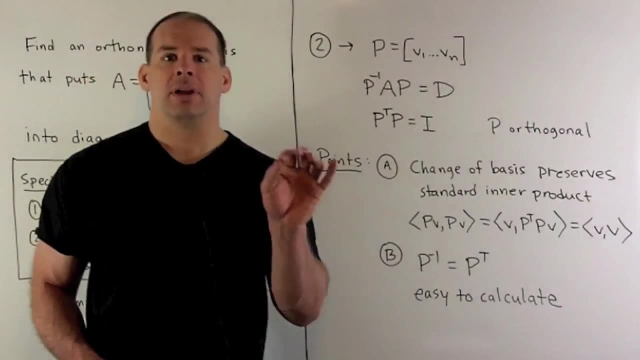 So what will that get us? First, it says that our change of basis is going to preserve the standard inner product. So if I start with lengths before I apply P, we're going to wind up having the same lengths after we apply P. 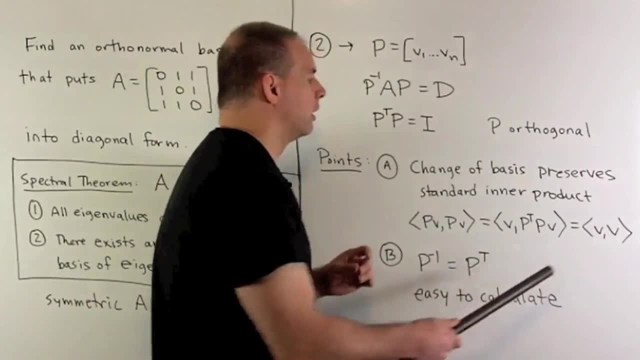 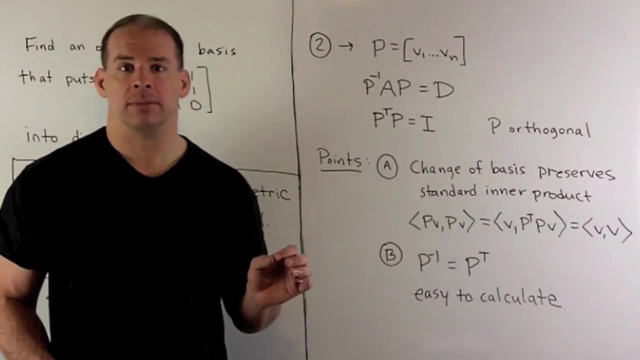 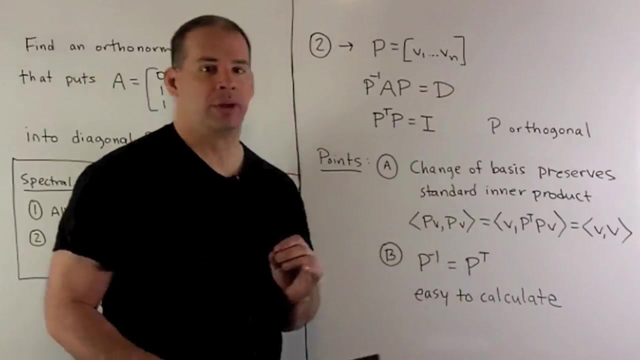 So that's all this says here. So the idea is our change of basis by: P preserves the standard inner product, It preserves angles and it preserves lengths, Then we'll also have that the inverse of the matrix P is just equal to the transpose. 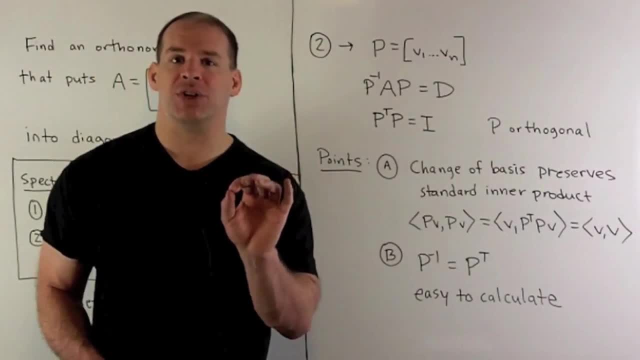 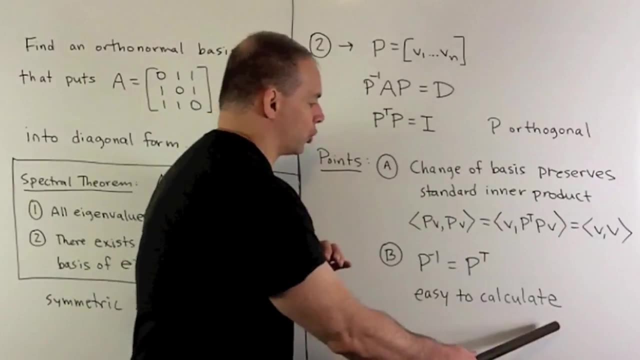 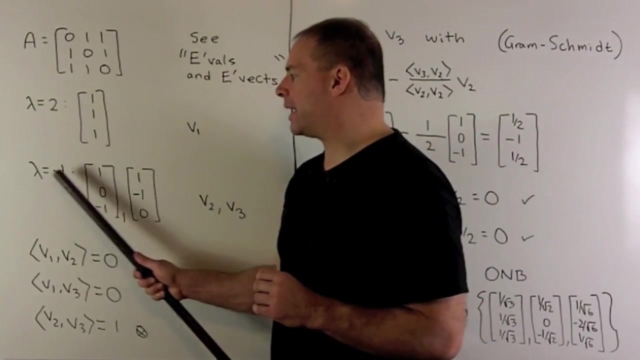 So from a calculation point of view it's much easier to take a transpose than it is to use our inverse formulas. So this is just a computational shortcut. For our matrix A, eigenvalues are going to be 2 and minus 1 with multiplicity 2.. 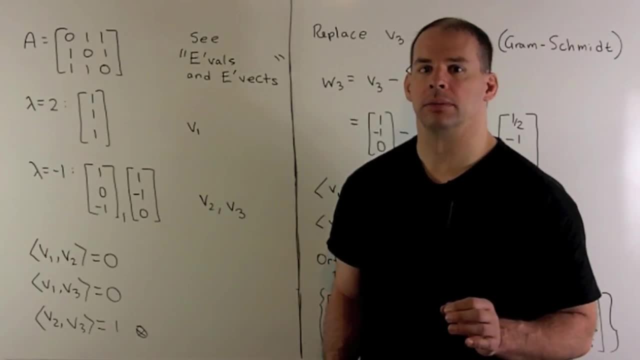 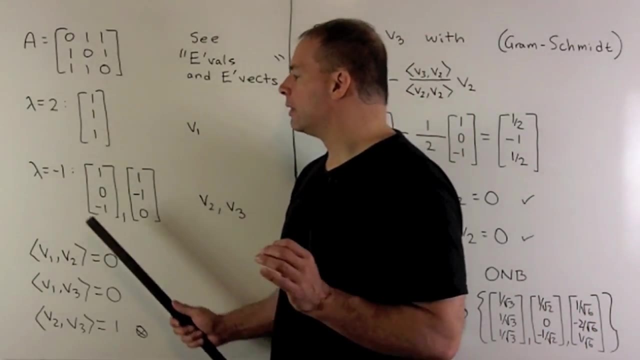 So that verifies that our eigenvalues are real For the corresponding basis of eigenvectors. for 2, we have 1, 1, 1.. For minus 1, we have 1, 0, minus 1,. 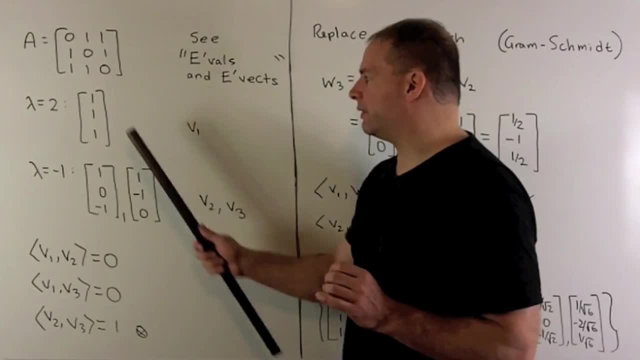 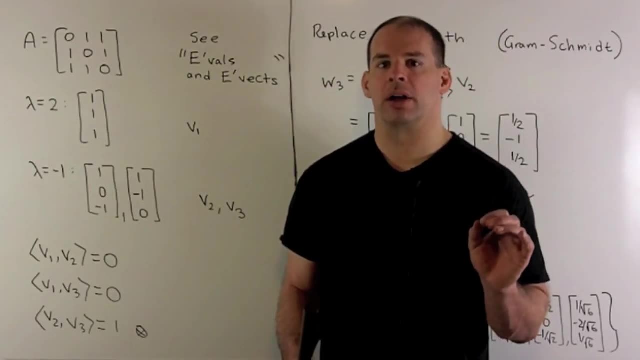 and 1, minus 1, 0. So we'll call these V1,, V2, and V3.. Now you should check those if you want to see the work that's in an earlier video. Eigenvalues and Eigenvectors. 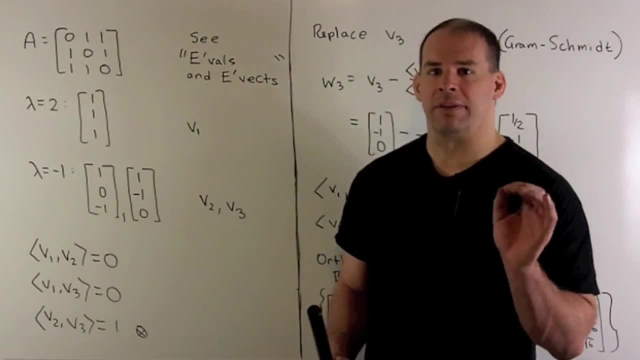 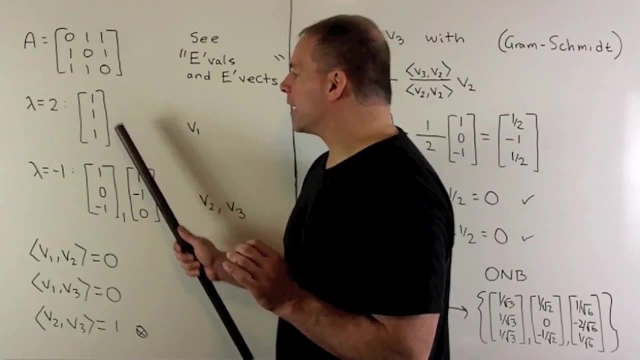 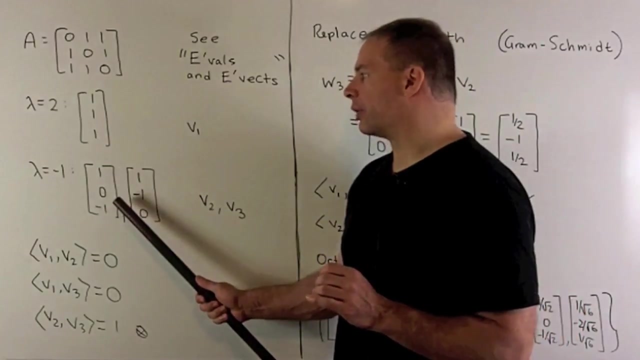 We want to show that we can find an orthonormal basis of eigenvectors. So let's see what we have here Now for eigenvectors corresponding to different eigenvalues. if you have a symmetric matrix, these are automatically going to be orthogonal. 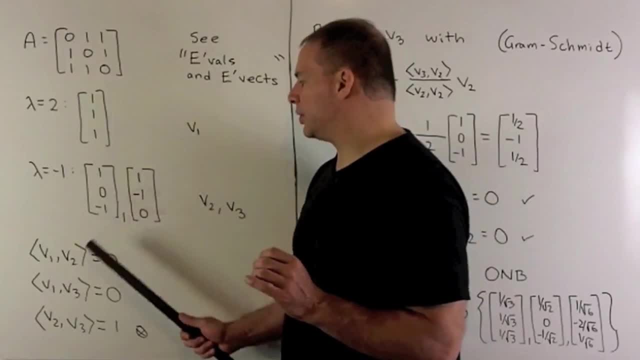 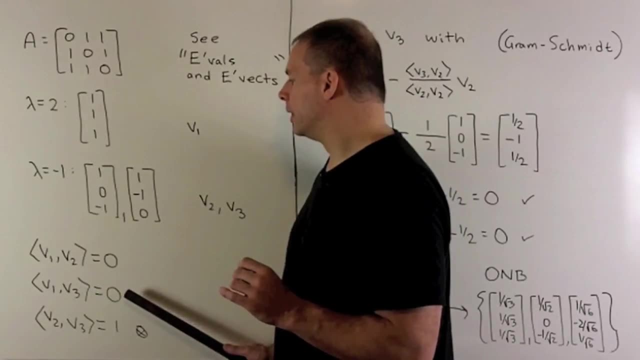 So let's check that. So if I take V1 against V2, I get a 0.. If I take V1 against V3, we also get 0.. If we take V2 against V3, I'm going to get a 1.. 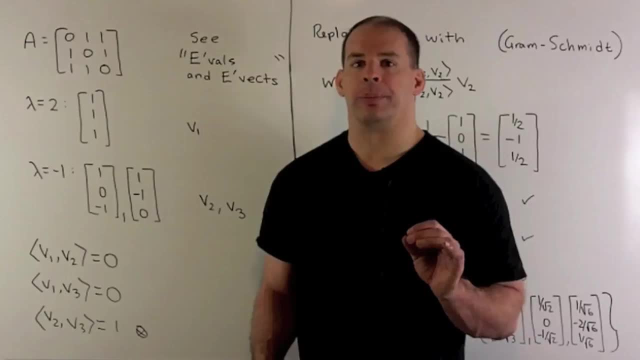 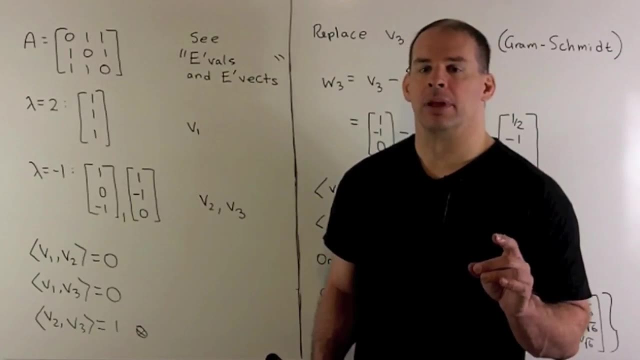 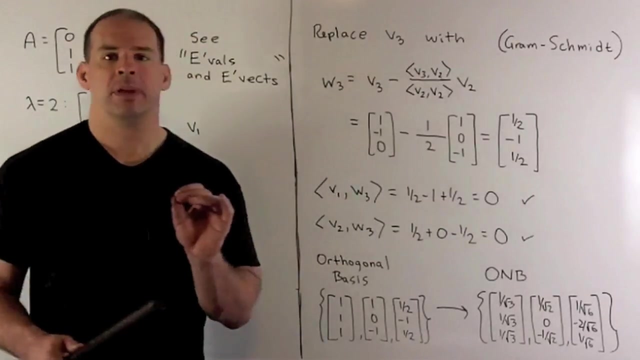 So our basis isn't orthogonal. We can make it orthogonal if we replace V3 with another vector. So what we'll do is we're going to replace V3 with W3.. Here we're going to take V3, subtract off the part of V3. 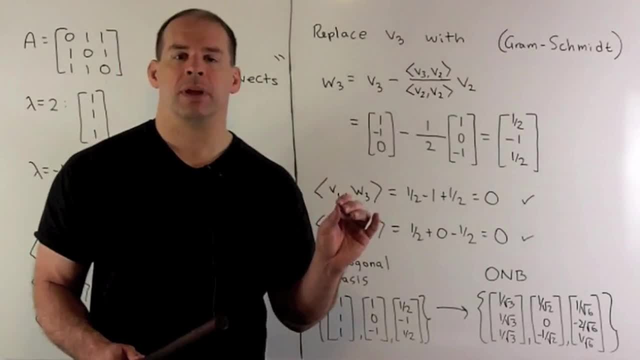 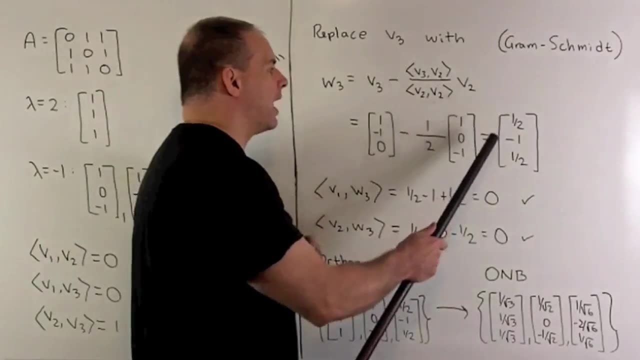 that's in the direction of V2.. Okay, we do that using a recipe. This is a recipe from Graham Schmidt. Now, when we work that out, we get the vector 1 half minus 1, 1 half If we recheck our inner products. 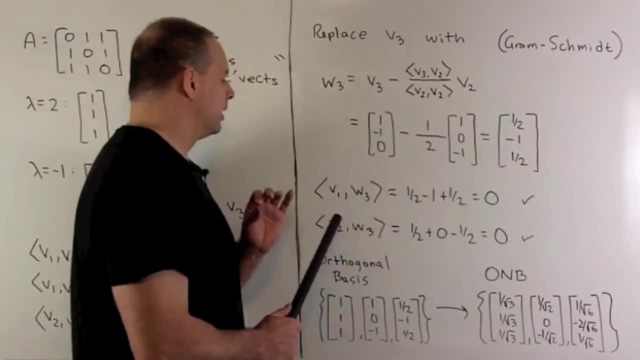 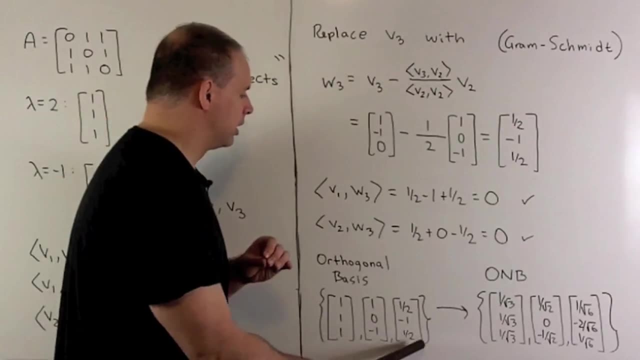 what will happen? well, V1 against W3 is going to be 0. V2 against W3 is also going to be 0. So now I have an orthogonal basis. To get an orthonormal basis, I just need to have unit vectors. 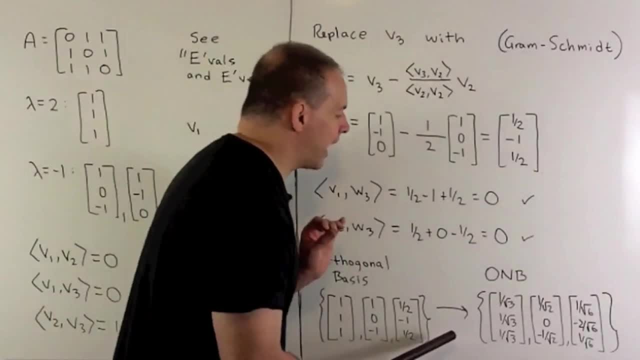 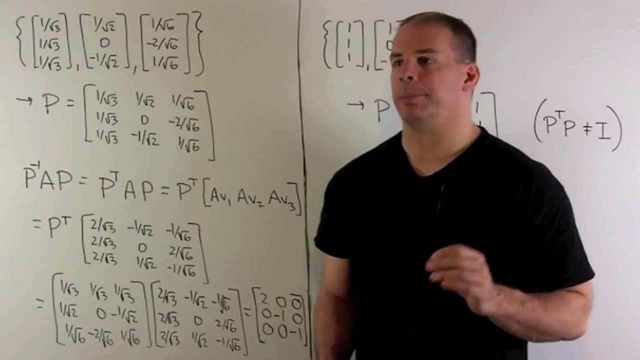 So we take each vector divide by its length. Then we have our orthonormal basis. over here Let's put our matrix in diagonal form. So we have our orthonormal basis. I'm going to load each basis vector in as a column of our matrix. 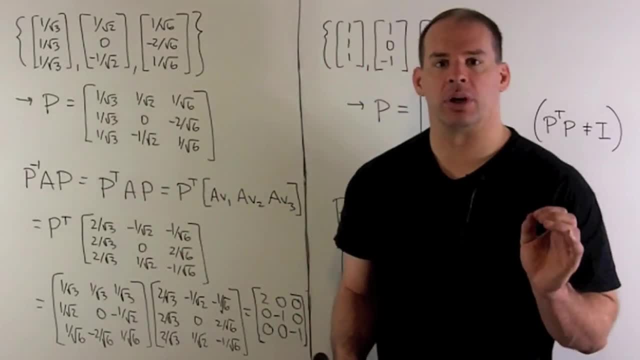 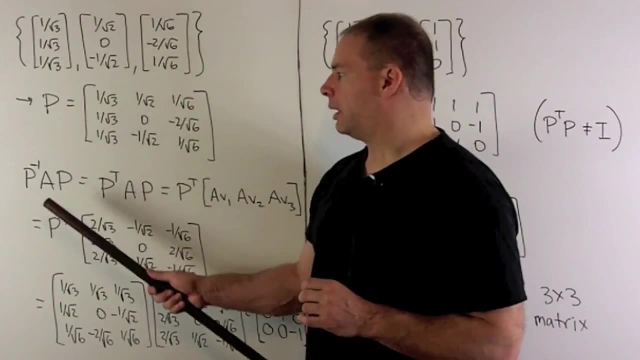 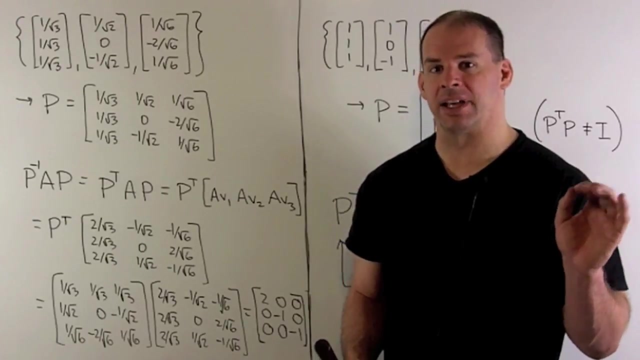 So we get our basis matrix P. Then we're going to compute P inverse AP. Now, since P is orthogonal, P inverse is equal to P transpose. Then I also have a transpose. This is a trick for multiplying A times P. 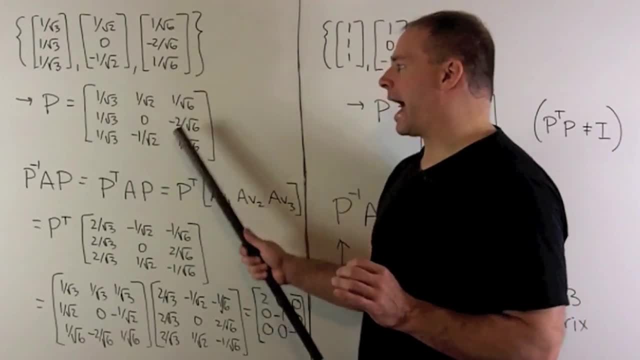 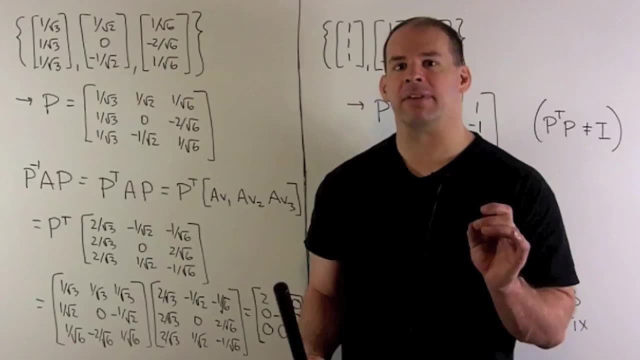 So for A times P. note that the columns of P are all eigenvectors. So if I multiply by A, I'm really multiplying each column vector by A, Since they're eigenvectors. we just multiply each column by the eigenvalue. 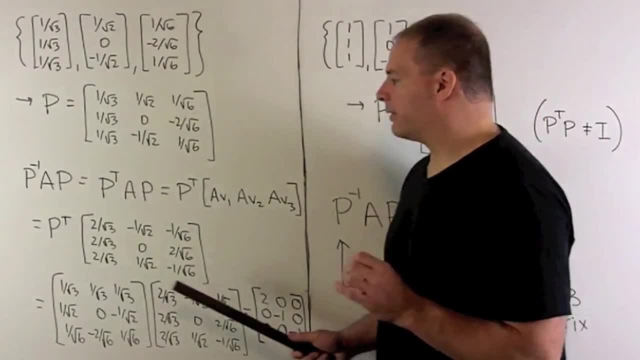 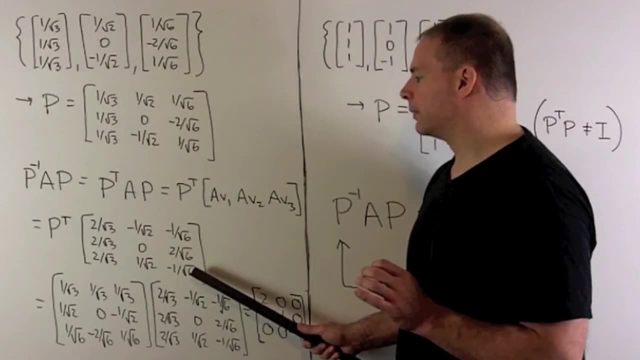 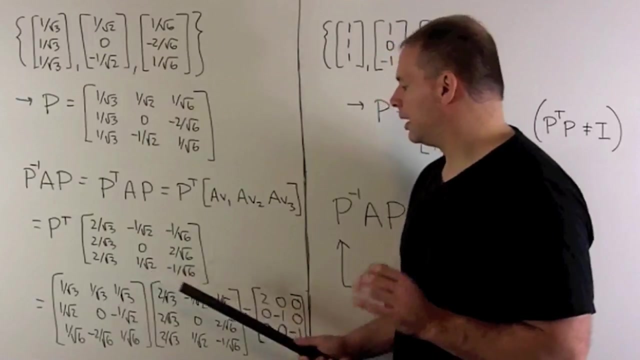 So for A times P we're going to have 2 times the first vector minus 1 times the second vector minus 1 times the third vector. Then we multiply by P, transpose. So we just flip our matrix across the diagonal, We work it out. 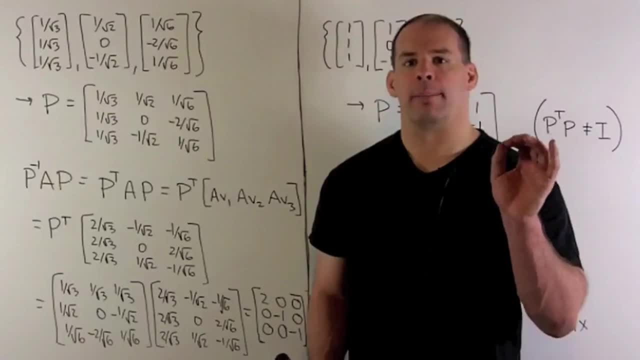 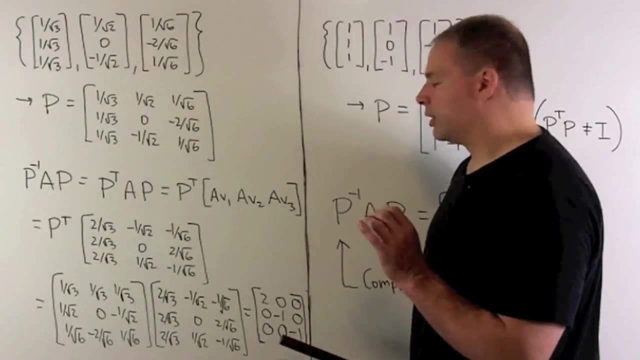 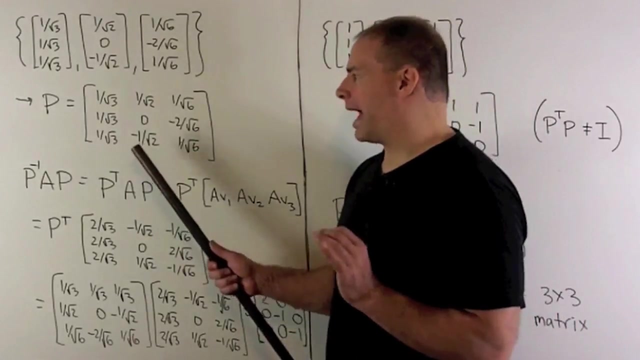 We get the diagonal matrix with entries 2, minus 1, minus 1 in the diagonal. Checking our work. These diagonal entries should be our eigenvalues, in the same order as our basis of eigenvectors. So here we're going to have 2, minus 1, minus 1..